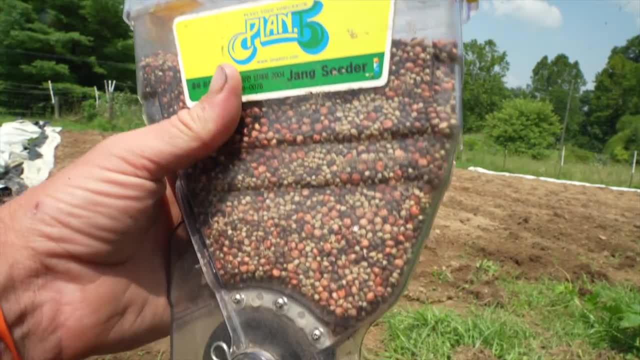 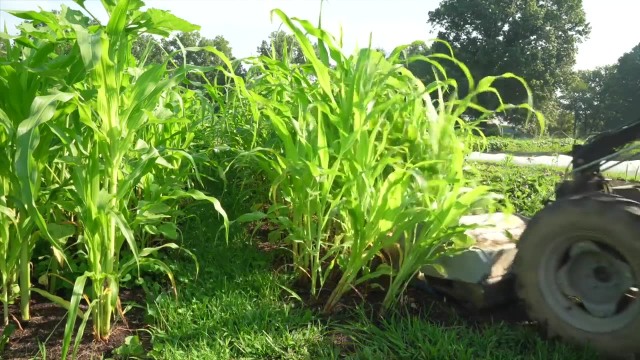 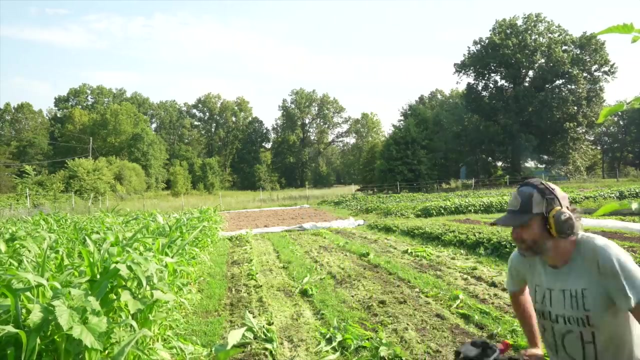 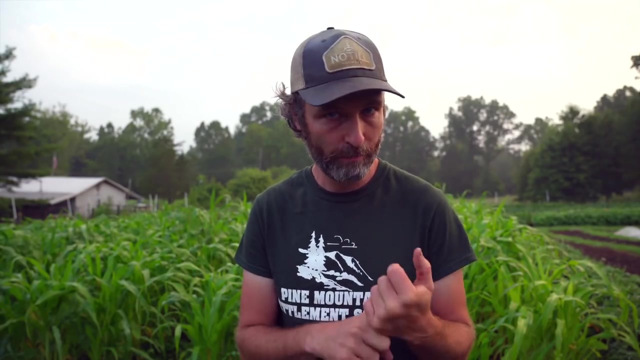 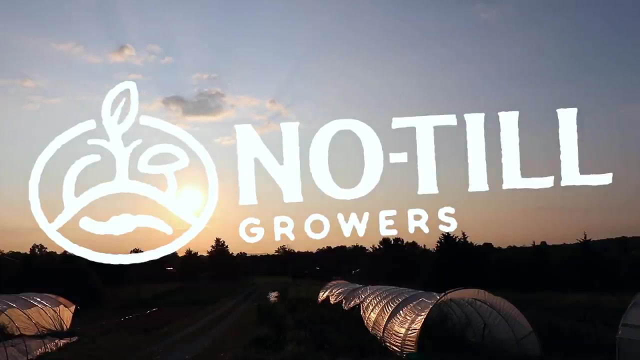 Hey you all, Farmer Jesse here. So today we're going to talk cover crops, Specifically choosing the right cover crop for what you need. So let's do it First things first. if you're not subscribed to this channel, make sure to hit the subscribe. 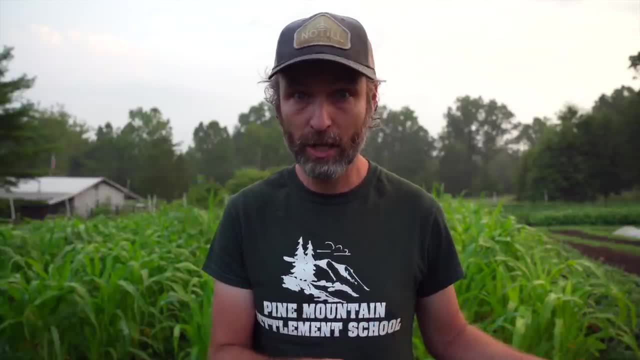 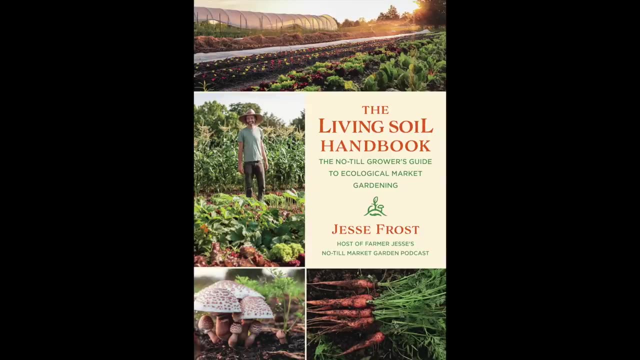 button And if you are subscribed, you're awesome. Second thing: I cover cover crops, cover cover crops. I cover cover crops a lot in my book, The Living Soil Handbook, which is on sale now. It is like out in the world, You can get it in Amazon and all those things. 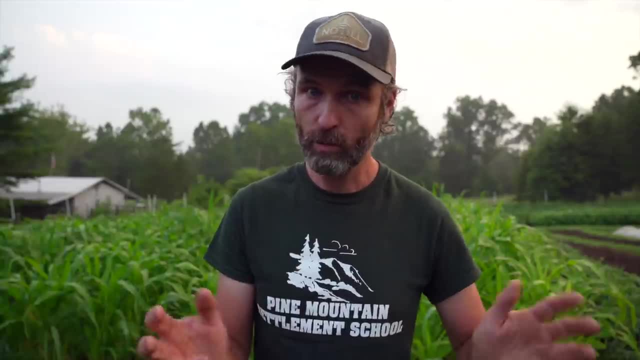 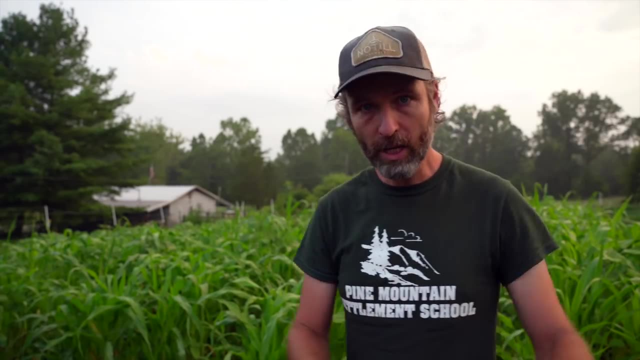 but preferably you'd get it from notillgrowerscom, because when you buy it there, the proceeds from that sale go to making more content for you, All right. So the real thing with cover crops is that you really have to decide what your goals are with it. Do you want? 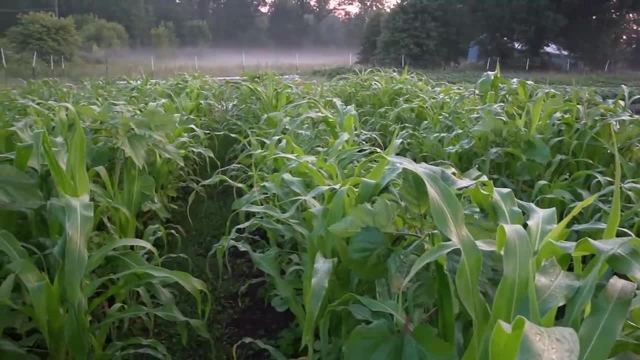 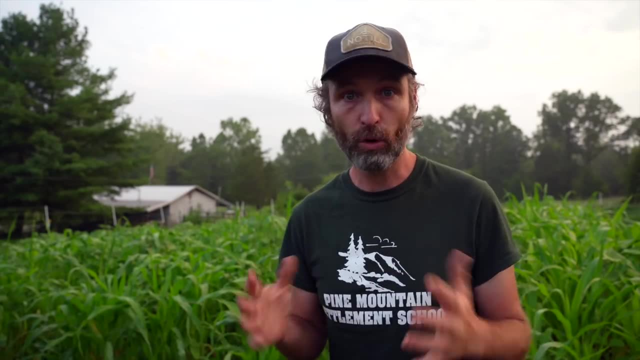 it as a mulch? Do you want it as a soil improver? Do you want it to just hold the place? hold your soil in place. Do you have four weeks in between one crop and the next crop that you just want something growing there as a placeholder? Lots of reasons to use cover crops, but not every cover. 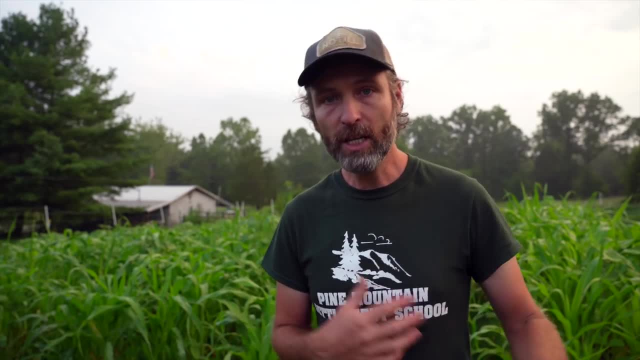 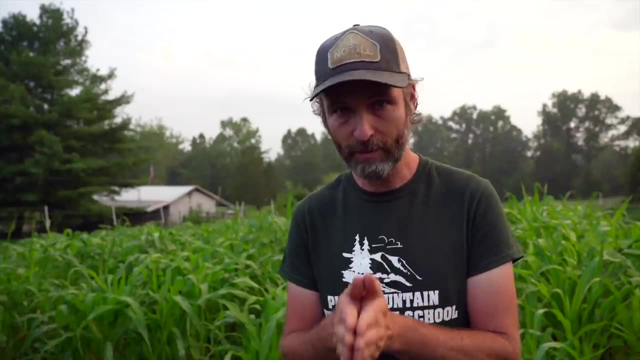 crop makes sense for every situation. So I kind of want to go through each of the individual reasons that you would use a cover crop and talk about which cover crops make the most sense in that scenario. And also, I do not have a monopoly On all the good advice or good ideas. I always want this channel to be collaborative. So 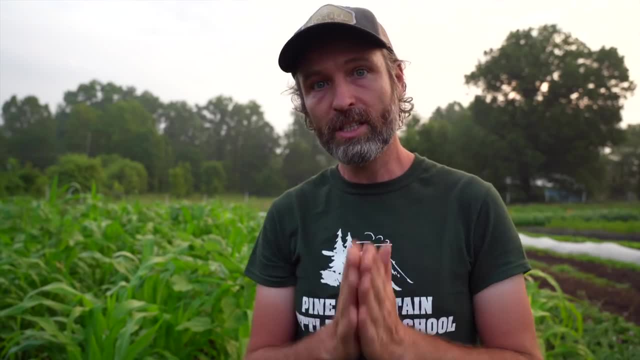 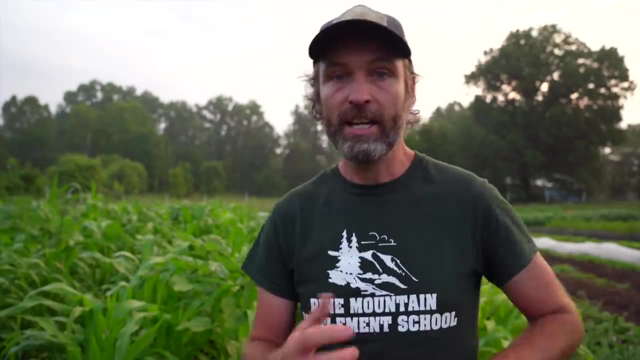 add your insight in the comments. One of the primary reasons people use cover crops is just for a mulch, a surface mulch. right, You can grow your mulch in place. Now there are cover crops that work really well for that And there are cover crops that don't work. 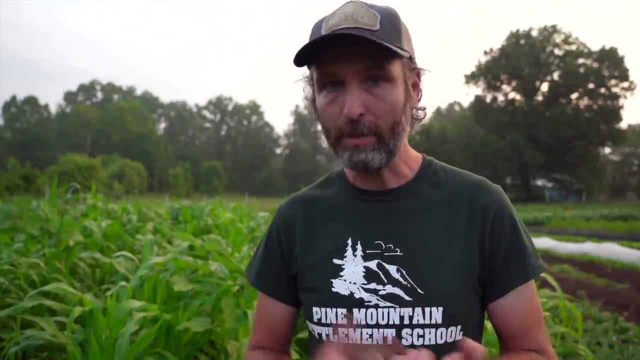 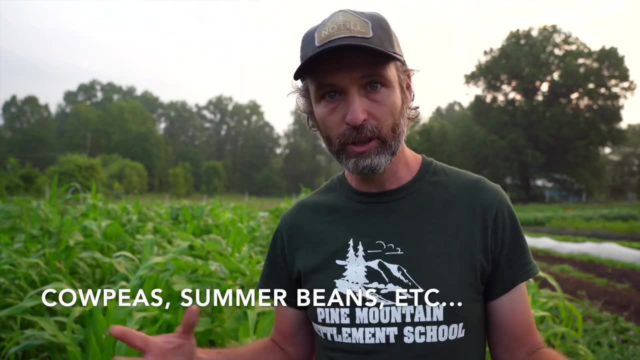 all that well for that. Generally speaking, things like beans, mung beans, soybeans, any of those- they don't make a great surface mulch. It doesn't last for a really long time. Things like buckwheat don't last for a very long time. They make like a very light mulch. 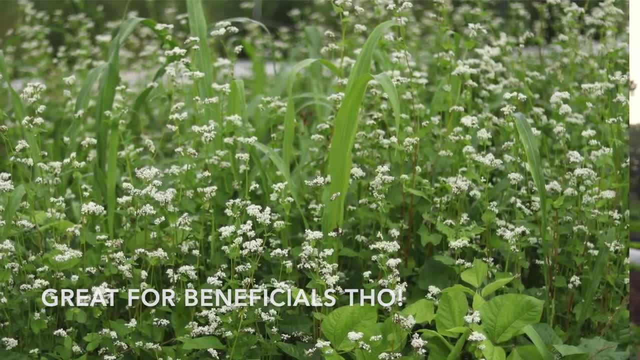 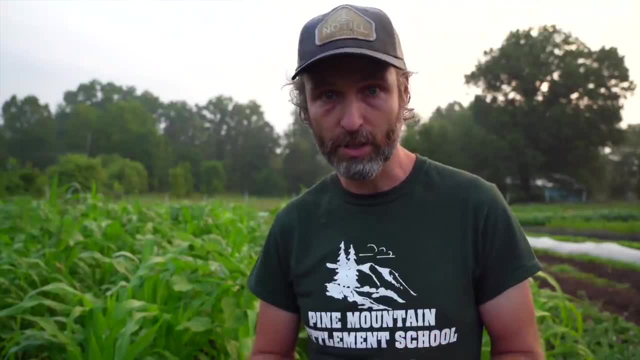 They're very succulent, very tender And they just kind of decompose really quickly. However, there are a lot of summer cover crops and winter cover crops that do make great mulches. So sorghum Sudan grass, for instance, is a really good winter mulch, a mulch for the winter. So 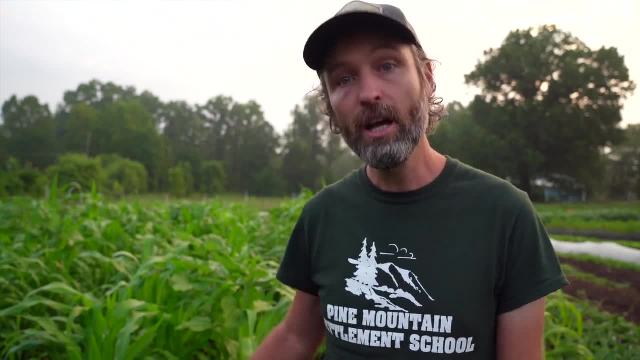 if you're going into the fall and you have space that you want to plant, for your fall planting, you could use something like sorghum. This isn't sorghum Sudan. I keep pointing to it but it's not. I'll talk about this in a second. But you could use something like sorghum Sudan. 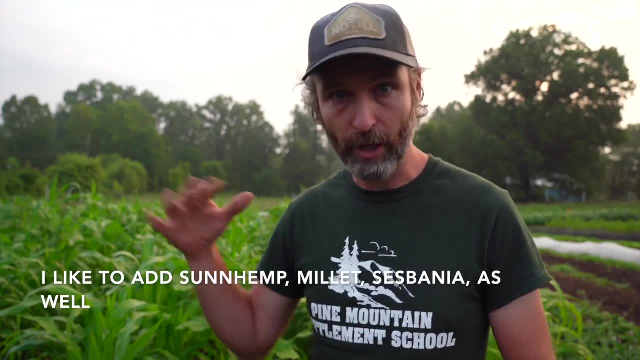 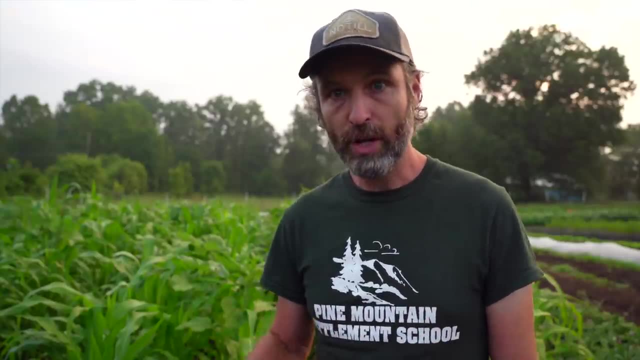 grass. It's a really good mulch for the winter. So if you're going into the fall and you have really great biomass above ground- and below ground creates a lot of soil, organic matter, just really good. extensive root systems So you can use something like sorghum, Sudan grass You. 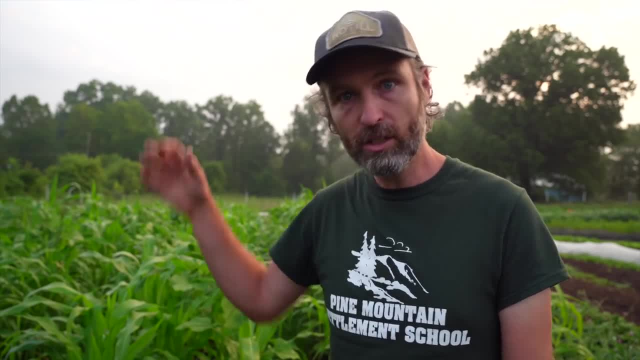 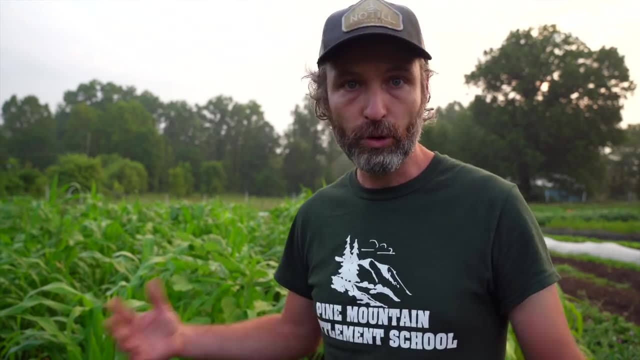 grow it really tall. Maybe you mow it a couple of times if you have the chance, And then when it gets really tall, right before frost, you can press it down. You can let it get frost or freezed. It will die. It's not a winter hardy cover crop, So something like that will create. 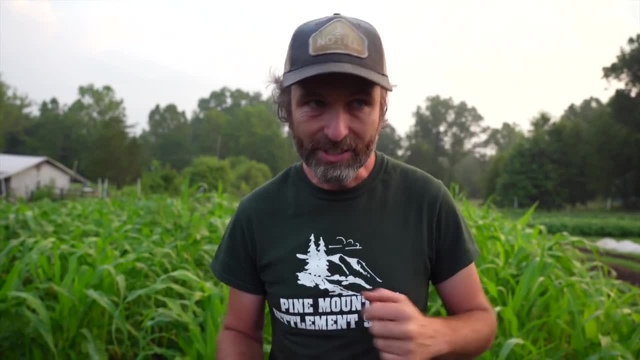 a nice mulch. You want a nice mulch going into the spring, So you would maybe use something like peas and oats that winter kill. Oats don't reliably winter kill in our region, So you may want to use something like that. So if you're going into the fall and you have space that you 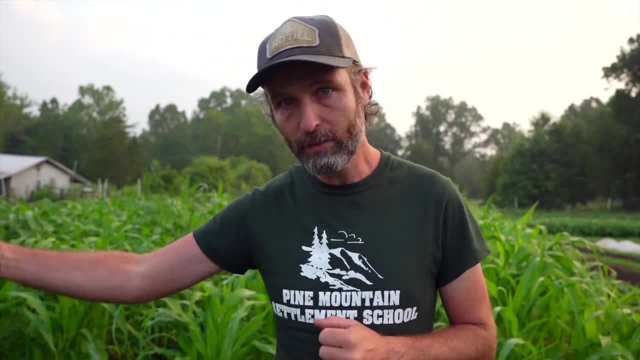 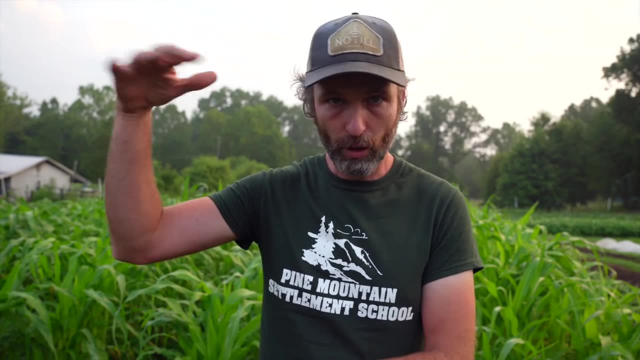 but something like peas and oats that grow pretty far into the fall, maybe even into the beginning of the winter, but are going to die after you get those first, like hard freezes. So that creates a nice above ground biomass and below ground, but for our purposes above ground, And then it gets. 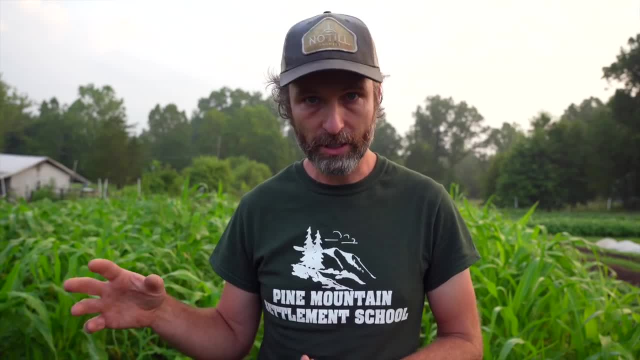 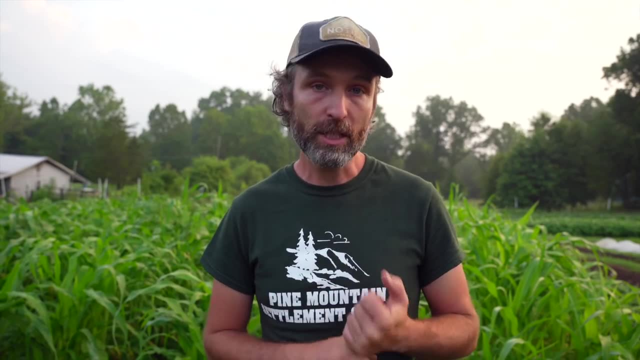 frozen, frosted enough times that the freeze thaw cycle ends up just wearing down the cell walls of the plant and it just breaks down. So it eventually dies and it creates a nice mat And that can be. that keeps it covered over the winter, keeps the soil in place over the winter, And then you can. 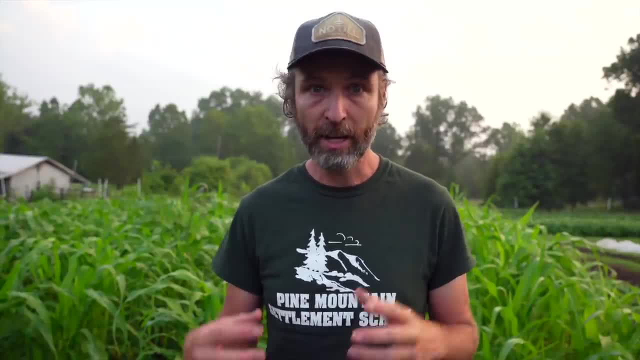 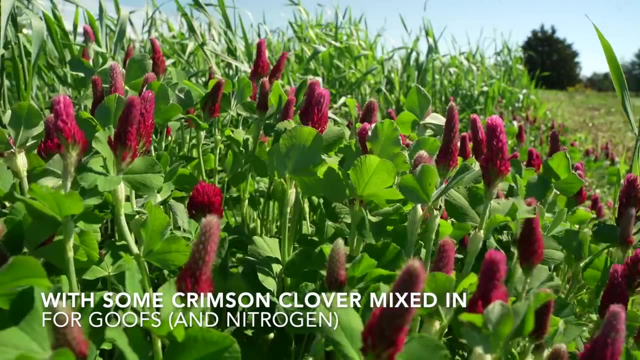 kind of rake that aside and plant into that in the spring, or just plant directly into that if you're doing transplants. However, that's not a super substantial mulch. A better mulch would be something like rye, vetch, wheat, some combination of those for the spring, So you let that grow. 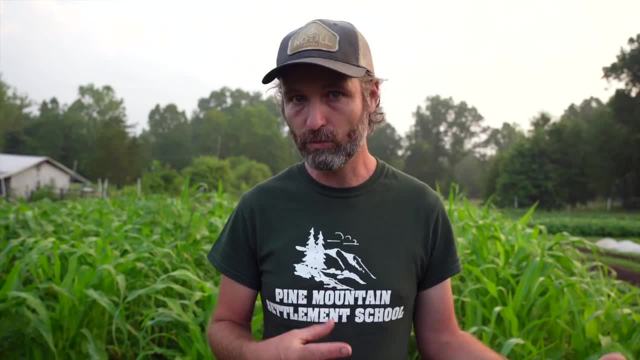 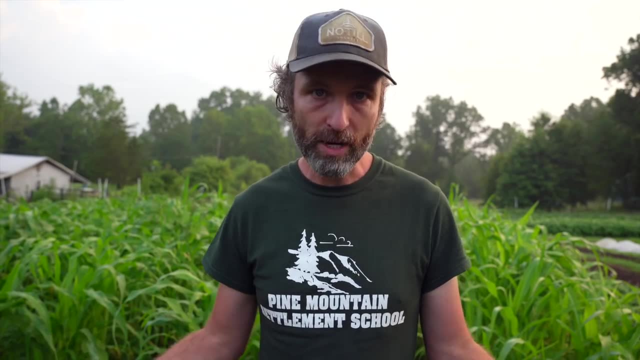 in the fall. It doesn't really die over the winter time in most regions, or a lot of regions, And then it kind of takes off in the spring and you press that down and you kill it in one of the many ways that you can kill cover crops- And I talk about crop termination in the book- And then 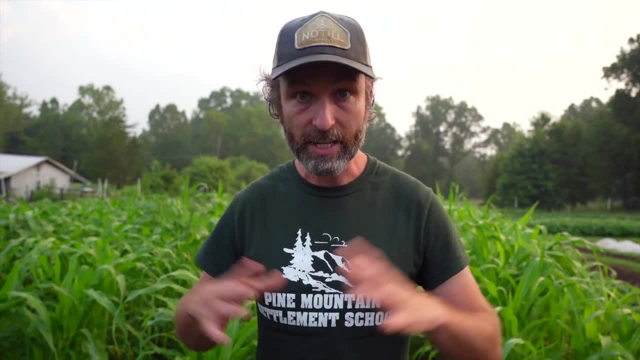 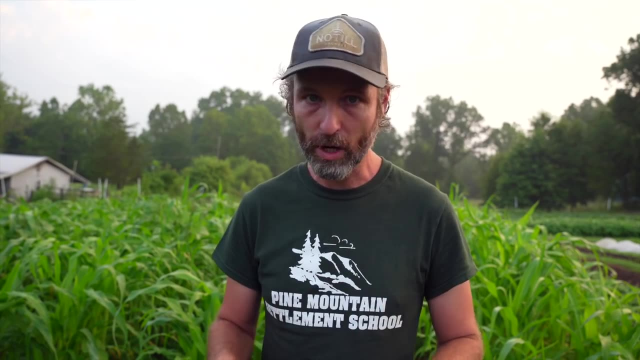 you press that down and effectively what you get is a nice mulch that lasts, you know, through most seasons. So in terms of mulches, those are like some easy options. Of course, there are a million ways to do this, So I'll try and cover as much as I can, but obviously it's a video, not a book. 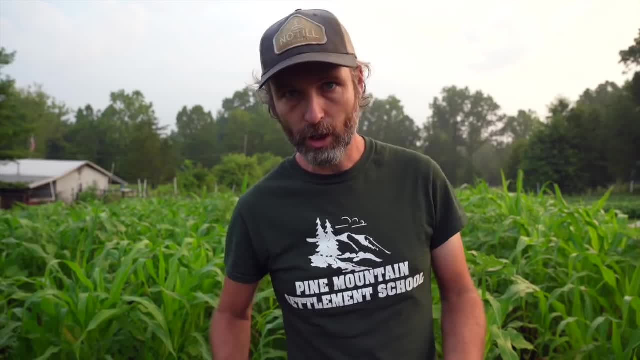 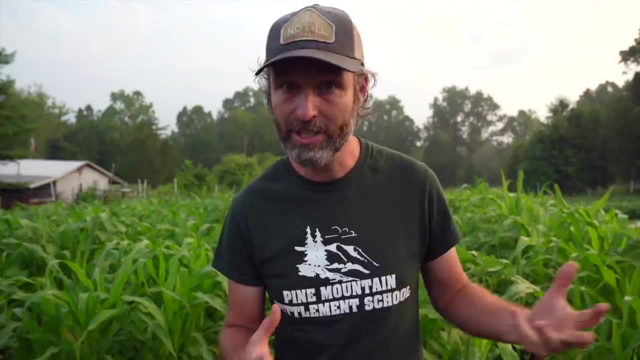 Anyway, and another popular reason for employing cover crops is for nutrients, for nitrogen in particular. Like legumes are really good at fixing nitrogen, as long as the rhizobium bacteria is present, They create those little root nodules. Those are where the nitrogen is fixed, because 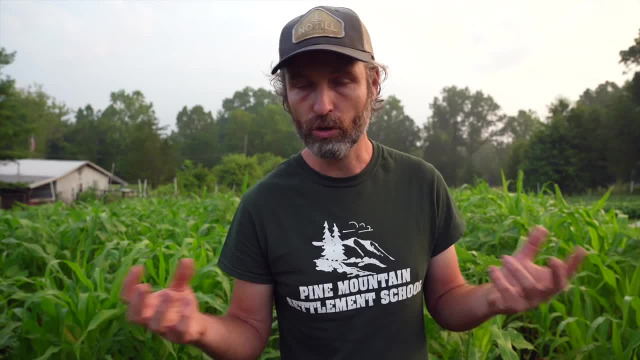 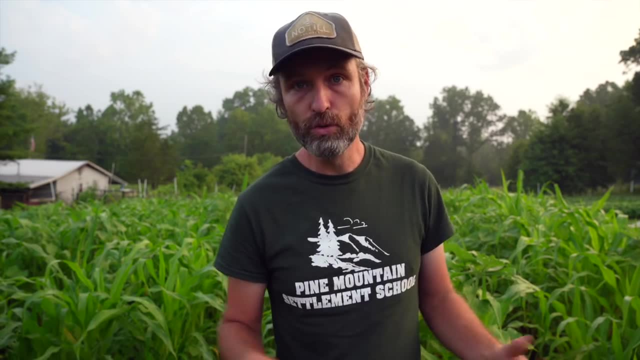 nitrogen fixation requires oxygen mitigation, like oxygen control, So these bacteria can actually use those little nodules to control oxygen intake and outtake, Anyway, so you can use these to gather nutrients, and they're gathering nutrients because they're photosynthesizing. So 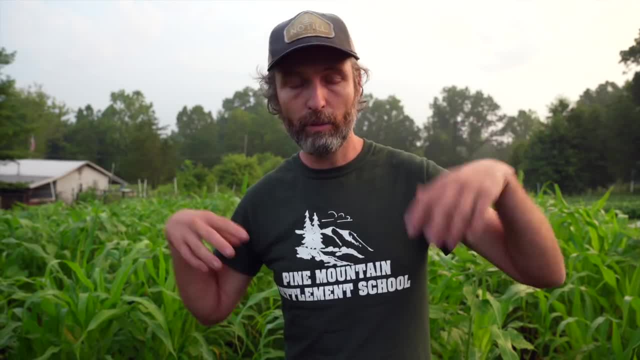 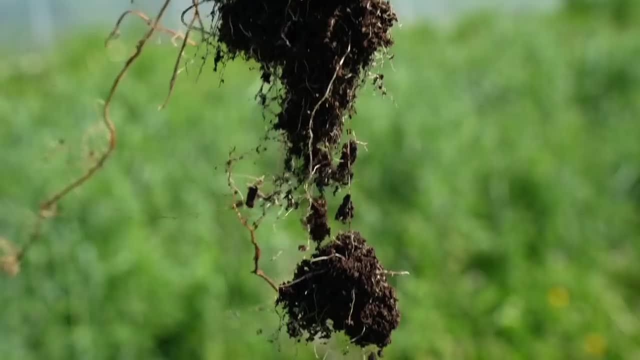 there's a nice green mat here bringing in carbon dioxide, sunlight and water and kind of mixing that together and creating glucose And that is feeding the soil So it's bringing in. each of these plants are bringing in a variety of different microbes that gather different nutrients, So like 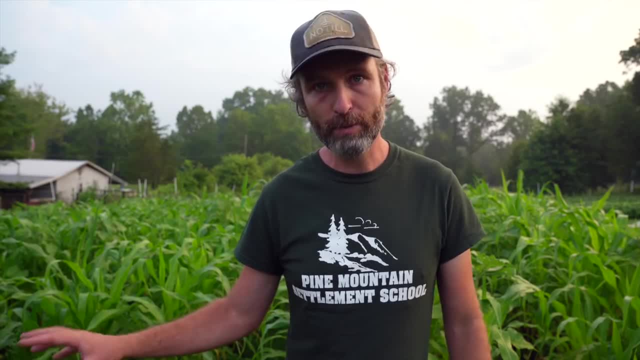 generally, you do want to mix. It's not just the legumes, Like, maybe you do want to pump some nitrogen in your soil, but you also want those other things. You also want to mix the different microbes that gather around in the different nutrients that they can collect. 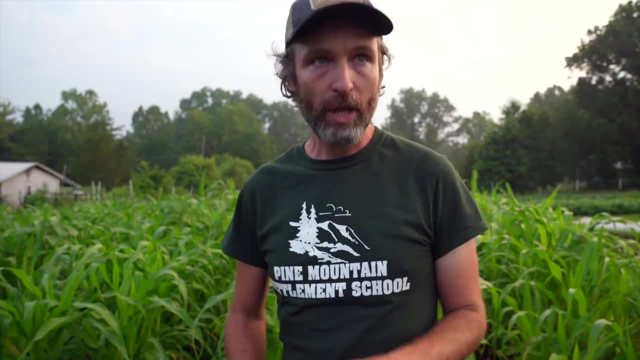 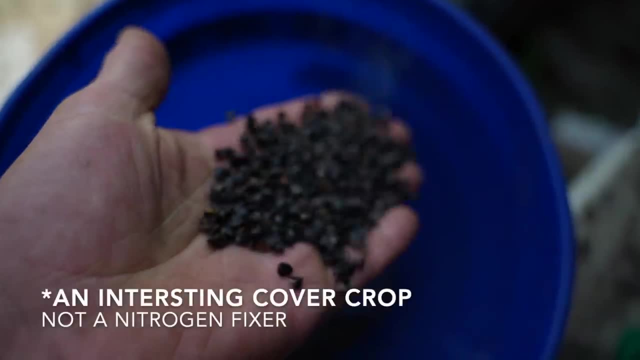 based on the variety of cover crops that you use. So that's anything in the legume family. pretty much is going to be a good nitrogen fixer, But buckwheat is a really interesting one too, because it's not doesn't have this like massive root system, but it is a really good gatherer of microbes and 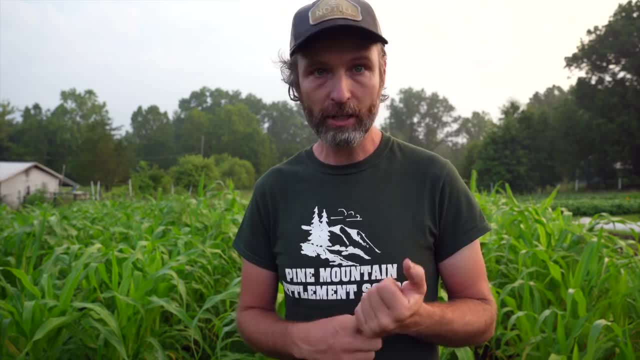 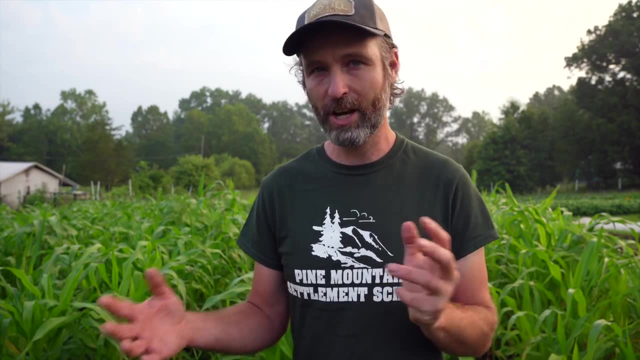 nutrients. You can also think of things like daikon radishes. Daikon radishes are often thought of as like a decompactor and they don't really do that. That's not, I mean, they kind of do. Studies are not really clear on whether or not they actually do that, So you can think of them as like a 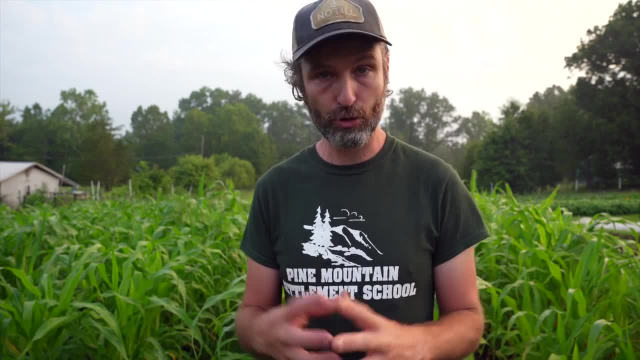 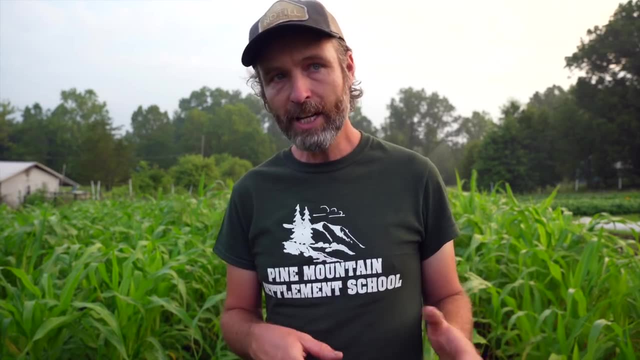 decompactor and they don't really do much decompaction, But anyway, what they do is they? they preserve nutrients, So they preserve a lot of nitrogen in the soil for the next crop in the next spring. And then there's also like allelopathic effects. This is sort of a weed management reason. 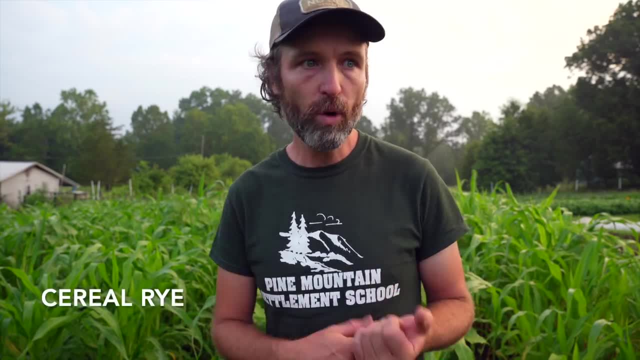 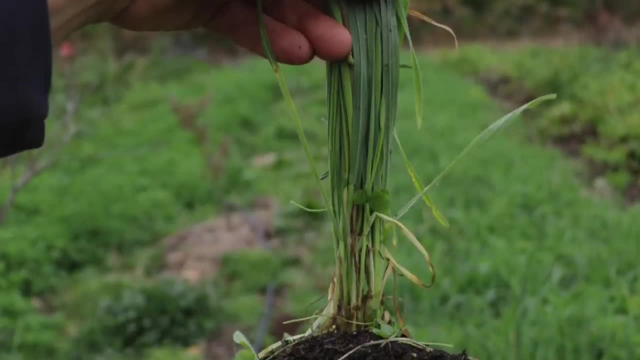 for using cover crops. So rye in particular is one, and so is sorghum, sudangrass and others that create an allelopathic effect. Essentially, the plants are creating specific chemicals to fight off weed germination. You know, often it's a specific plant, like other grasses, but generally 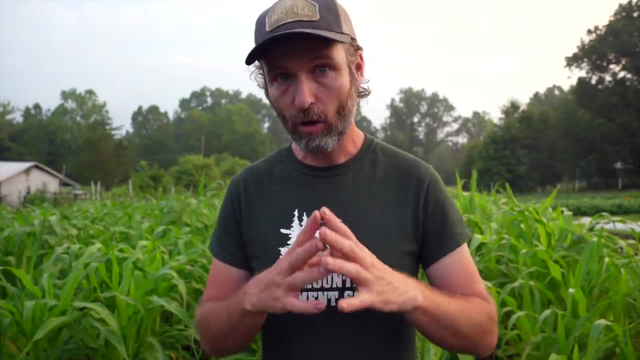 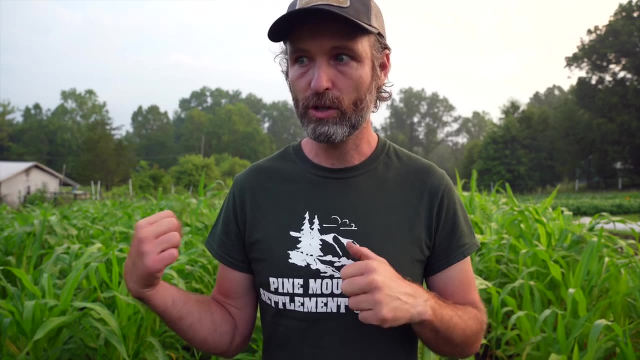 they're creating these specific chemicals that are going to fight off weed germination. So they're creating specific chemicals that are reducing growth of other plants and also reducing the germination rates of those other plants. So you can actually also use cover crops just to help with weed control, and not just in the mulch but, like I said, in those chemicals. 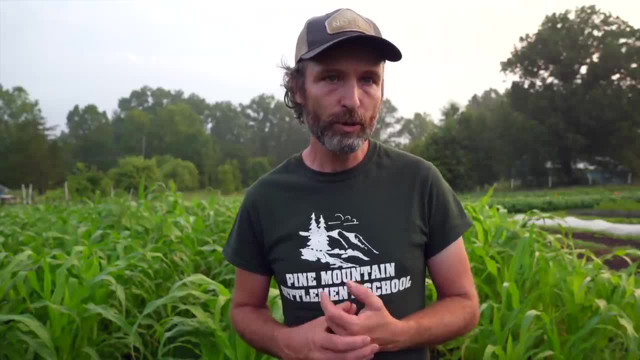 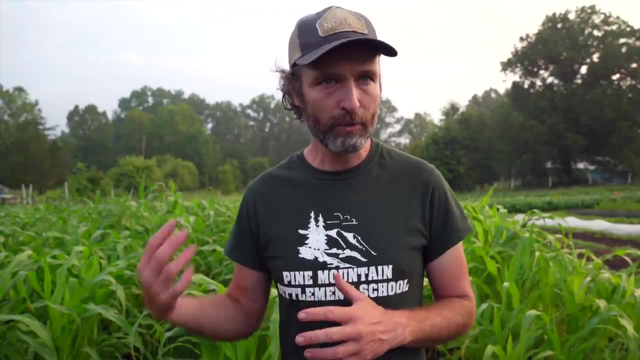 And there's also things like biofumigation. This one's not super clear to me how effective it is, because healthier soil is going to be less prone to disease And if you're growing a lot of cover crops, you're going to get healthier soil that has, you know, more nutrients. 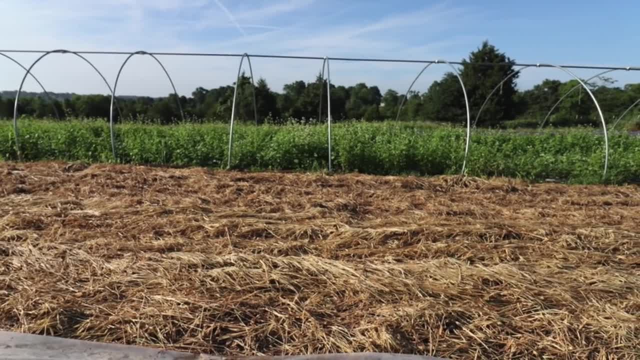 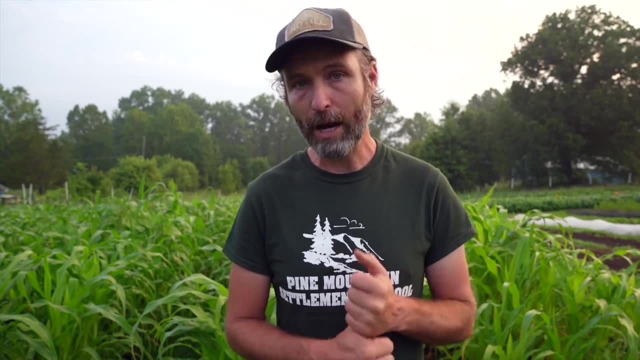 gathered and more you know, better tilth and more soil that's going to be able to grow soil, organic matter and all the things. But people have had some amount of success reducing certain bacterial wilts and fungal diseases using biofumigants, And these are essentially 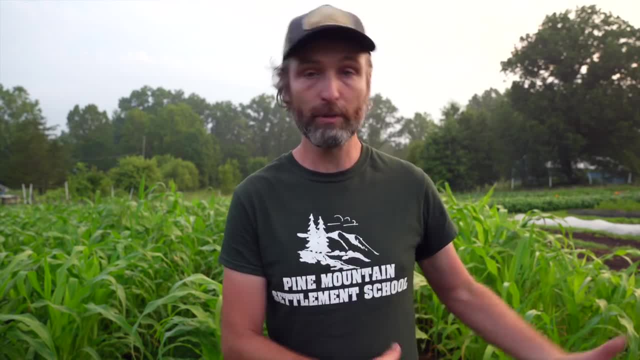 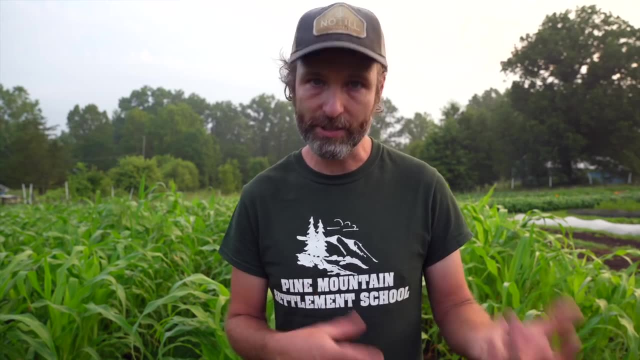 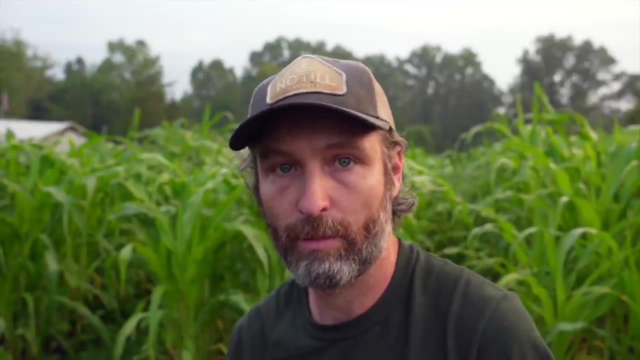 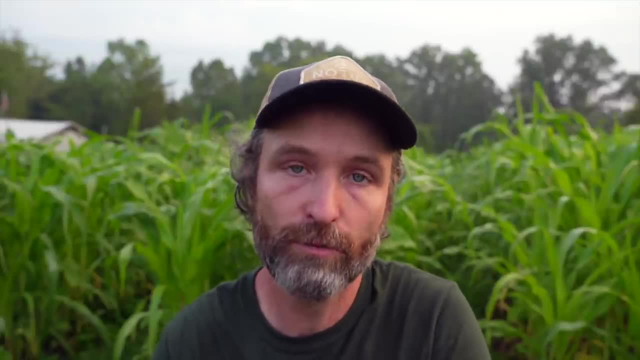 organic matter is a big reason why you would grow soil organic matter. Soil organic matter is a big reason why you would grow soil organic matter. Soil organic matter is a big reason. roller crimping as a way of terminating- and not every crop is going to be easy to terminate that-